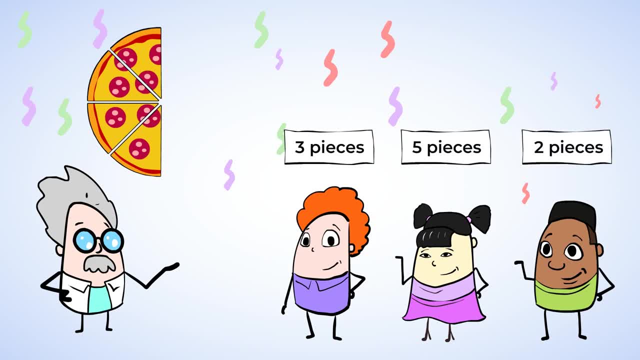 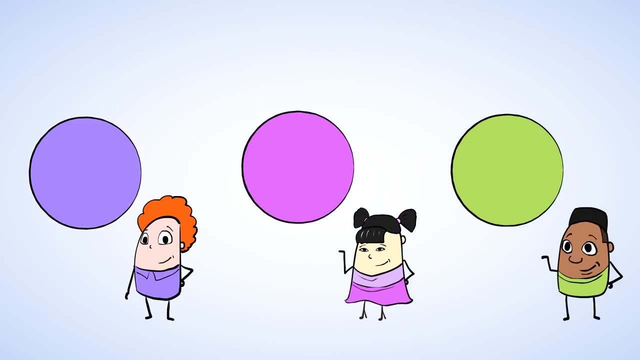 Courtney ate five pieces and Juan ate two pieces. Huh, How is that possible? Let's visualize it. Okay. here we have the three pizzas And we can split them in half, since we know each of them ate only one half. Tim ate three pieces, so we can split the eaten half into. 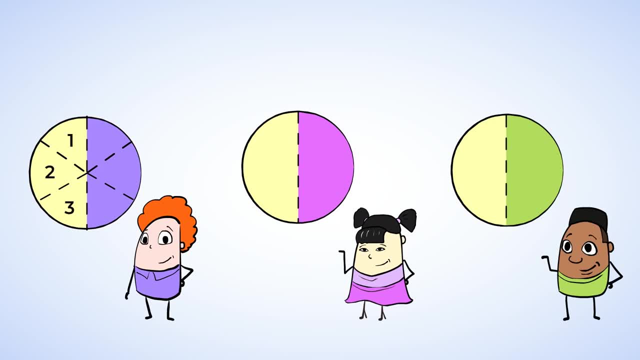 three pieces: One, two, three And the uneaten half can also be split into three pieces. It looks like Tim cut his pizza into sixths and ate three-sixths of the pizza. Now let's do the same with Courtney's pizza. 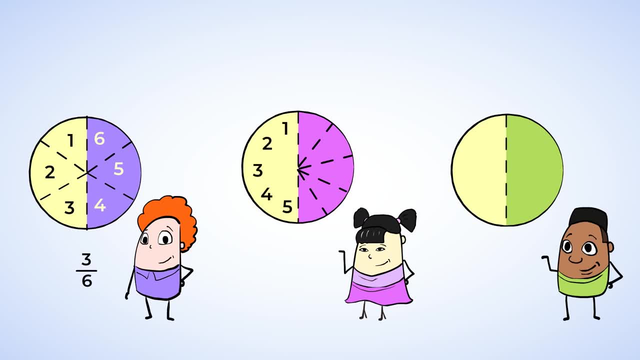 Now remember, she ate five pieces. If each half of the pizza got cut into five pieces, well then, there's a total of ten pieces. She ate five-tenths of her pizza And Juan only ate two pieces, which means that he ate two-fourths of his pizza. 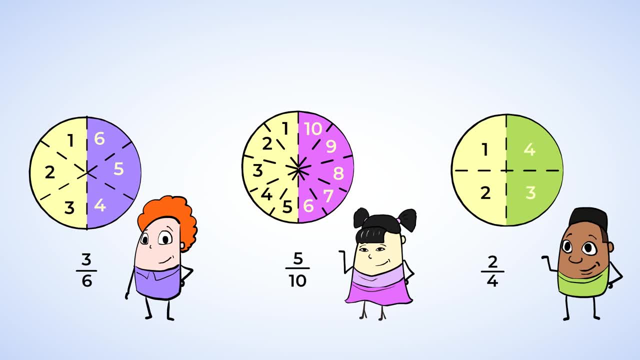 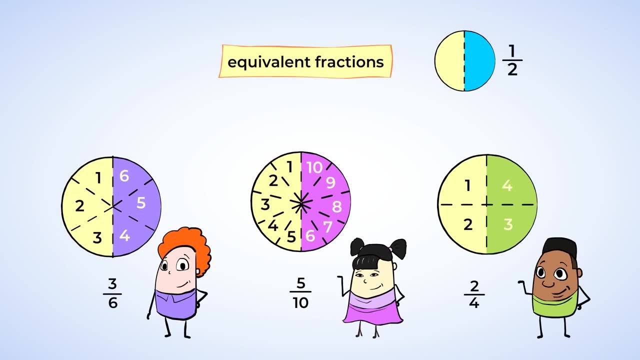 Although each of these fractions look different, we can see that they all represent the same amount: One half. These are called equivalent fractions. The word equivalent means equal in value. Equivalent fractions may have different numbers, but the value of the fractions is all the same. 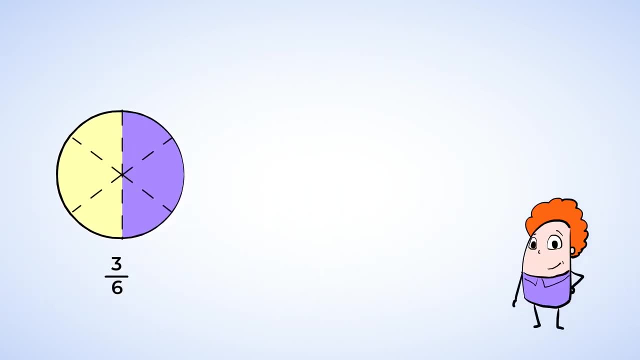 Let's look at how one half can become all of these different fractions. Tim ate three out of six pieces. We can change the fraction one half into three-sixths by multiplying both the numerator and denominator by three. One half times three-thirds equals three-sixths. 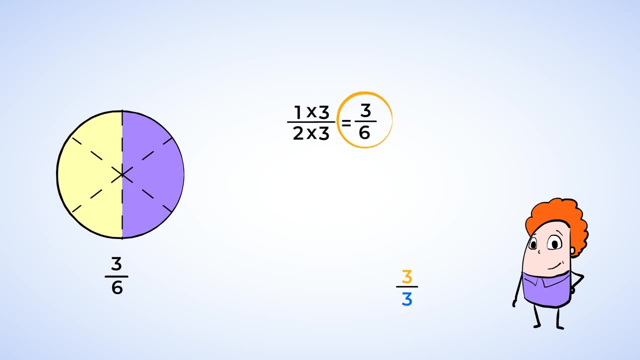 Remember, if the numerator and denominator are both the same number, it is equal to one. Now, you've just multiplied one half by three-thirds, which is equal to one, And if you multiply a number by one, it doesn't change, does it? 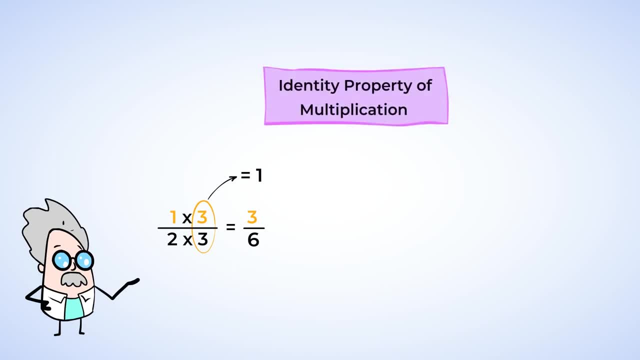 Now, that's a fancy property called the identity property of multiplication, which basically states that multiplying any number by one gives you that same number. You probably already knew that, but now you know the fancy name for it. Now let's do the same for the rest of the fractions. 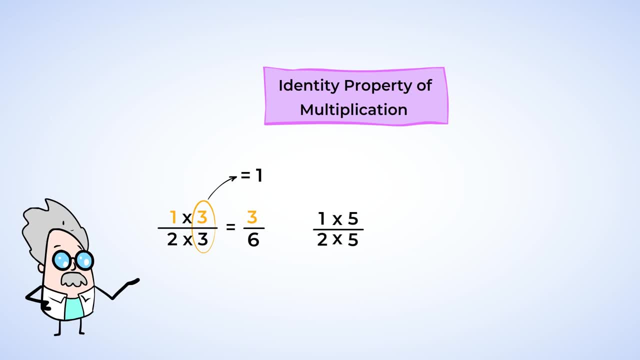 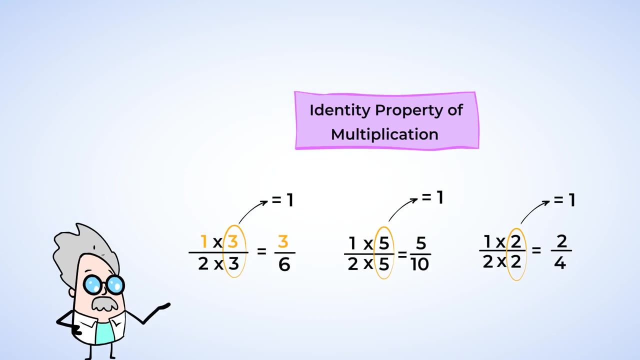 We can multiply one half by five-fifths to get the new fraction of five-tenths. And if I multiply one half by two halves, the result now is two-fourths. Now check this out. It brings us right back to the beginning of the story. 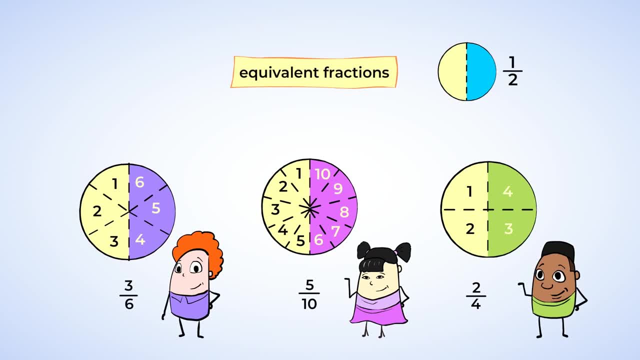 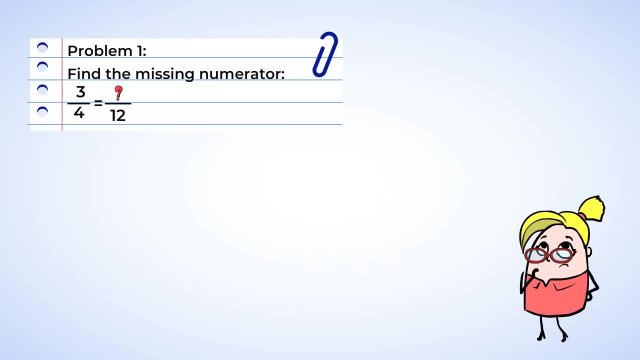 All three of these new fractions are equal to one-half. Cool, we just made some equivalent fractions. Find the missing numerator. Okay, looks like we have to find the missing numerator Now. the key with creating equivalent fractions is to multiply both the numerator and denominator. 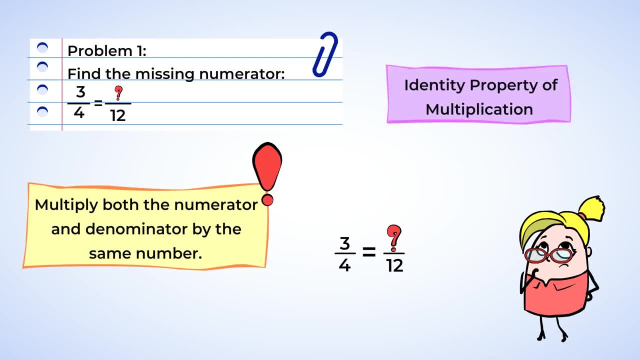 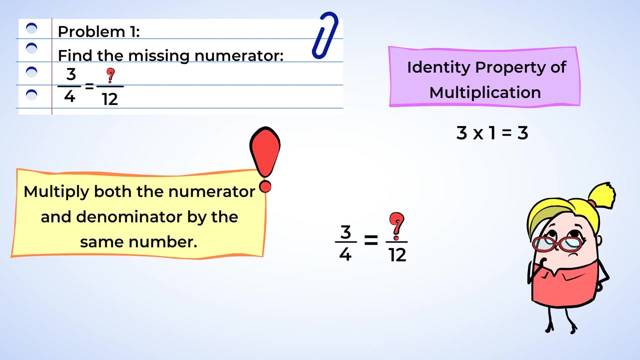 by the same number. That's because the identity property of multiplication lets us change the numbers of a fraction without changing the actual value. Remember that anything times one is itself right. So, looking at the denominators, what did we multiply four by to get twelve? 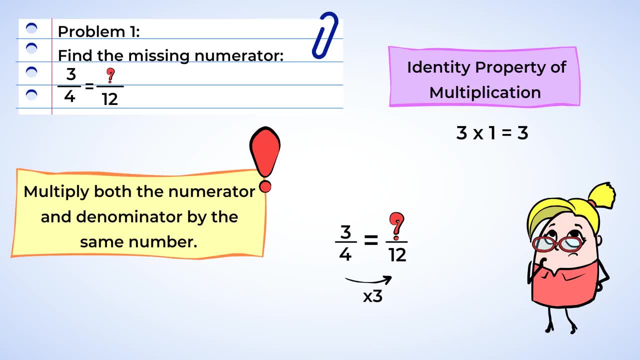 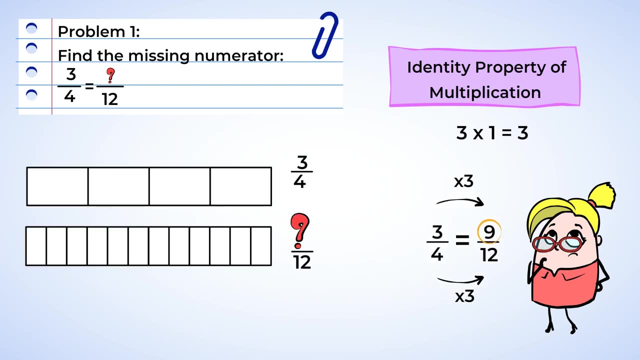 Four times three is twelve, so it's three. Whatever we do to the denominator, we need to do to the numerator. Three multiplied by three is nine, so that gives us nine-twelfths. The missing value Is nine. Now, just to be safe, let's draw out these fractions to help us show that we're correct. 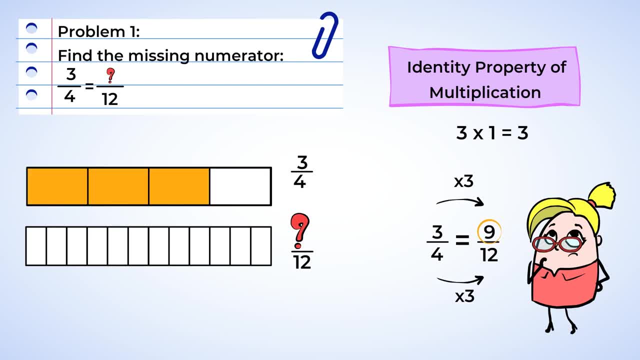 We know that three-fourths has four parts, with three that are shaded in. We also know that the second fraction has twelve total parts and we need to find out how many are shaded. And now we can shade in the same amount for the second fraction and if we draw a line, 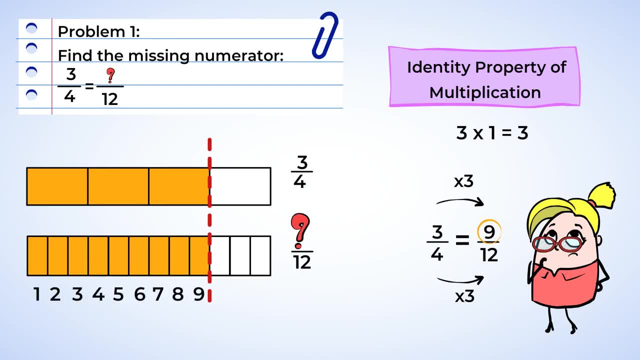 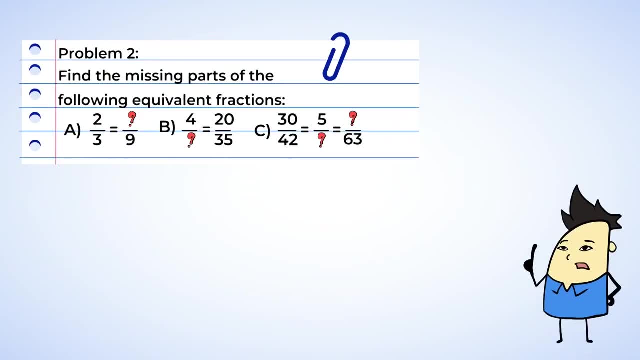 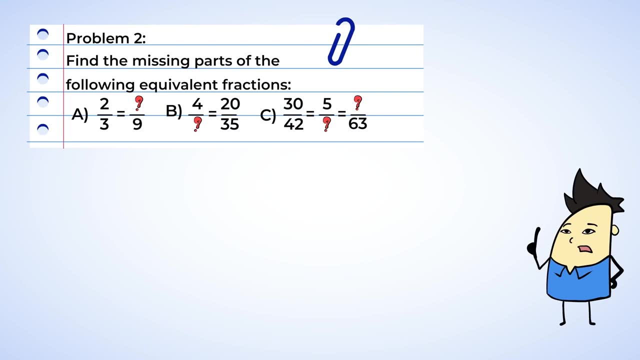 down. we can see we need to shade in nine parts. Looks like the multiplication we did was fantastic. Great job. Now let's keep it going with these equivalent fractions. Okay, we need to find the missing parts of the following equivalent fractions: 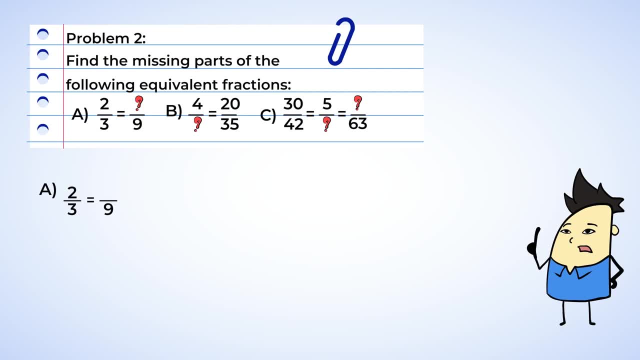 Let's start with part A. Since both fractions have denominators, let's see how we can use multiplication to get from three to nine. Okay, we multiply by three. Whatever we do to the denominator, we need to do to the numerator. 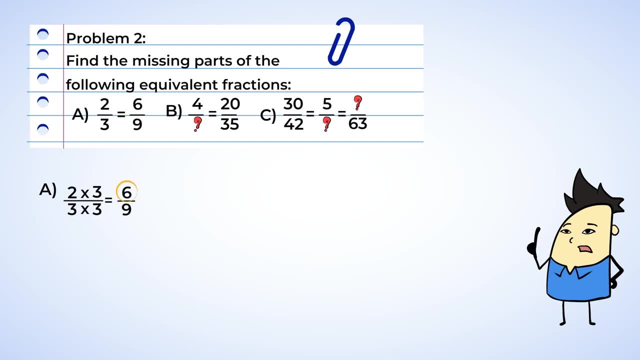 Two times three is six. Ah, Six is the missing number, and two-thirds is equal to six-ninths. Okay, moving on to part B. Now. this example has both numerators, and so four times what is twenty Five? 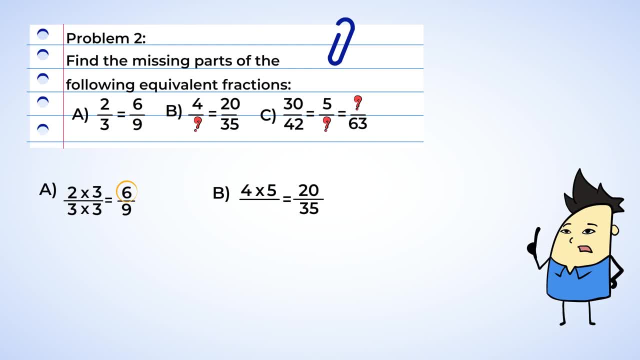 Since we needed to multiply the numerator by five, we also have to multiply the denominator. We need to multiply the denominator by five. We need to multiply the denominator by five as well. And what times? five is thirty-five, Well, seven, The denominator is seven. 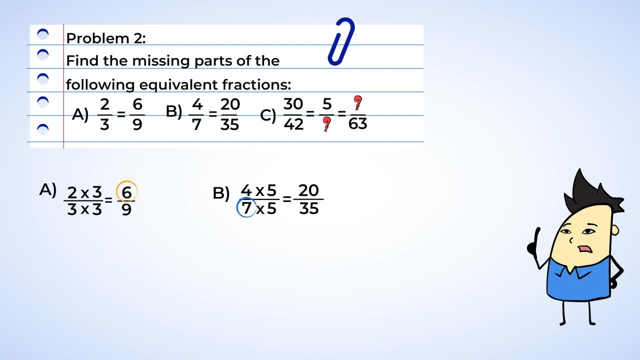 We could have also used division to find that answer as well, couldn't we? Thirty-five divided by five is seven. Huh, How neat. Okay, next up, part C: Whoa, This one has two unknown numbers. Looking at the numerators, how do we get from thirty to five? 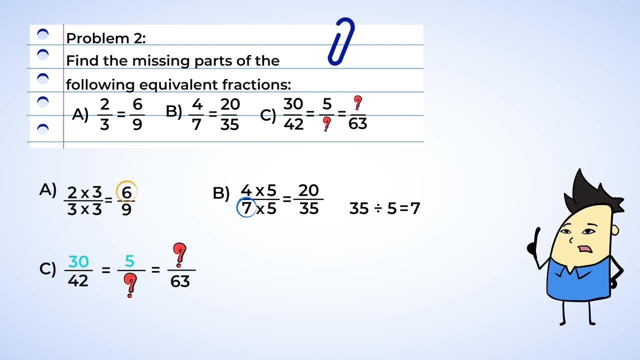 Okay, since the numbers get smaller, instead of multiplying, it looks like we're dividing. Thirty divided by six gives us five, and so that means we can divide forty-two by six to find our missing denominator. Forty-two divided by six is seven. 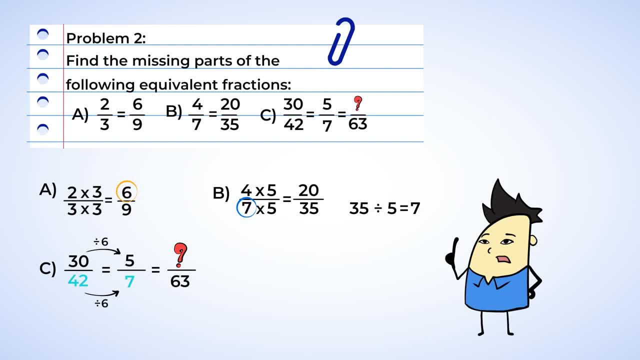 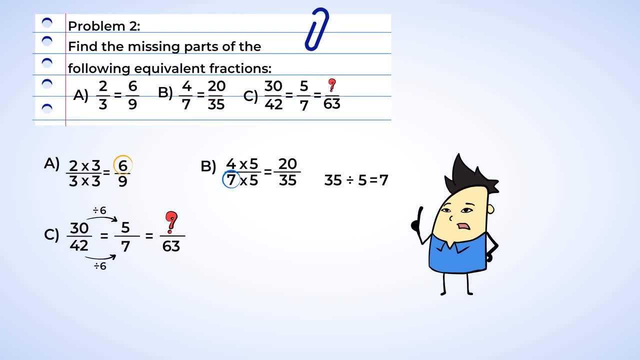 All right, we found that the fraction thirty-forty-seconds is equal to five-sevenths. but let's pause for a second and think about what we just did. Okay, First time we divided a number to make an equivalent fraction. 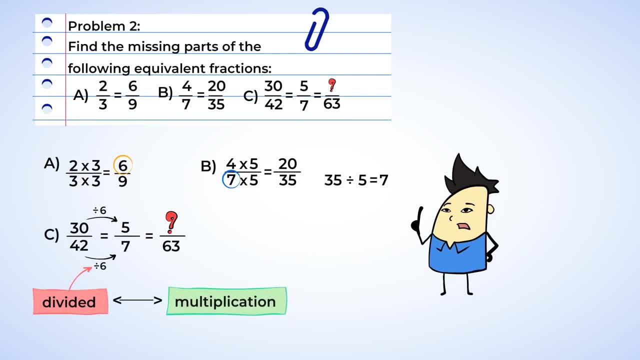 Now just remember: multiplication and division are very closely related. They're inverses or opposites. Now we can use the identity property of multiplication to multiply a fraction by one without changing its value, And we can also divide a fraction by one without changing its value, thanks to the identity. 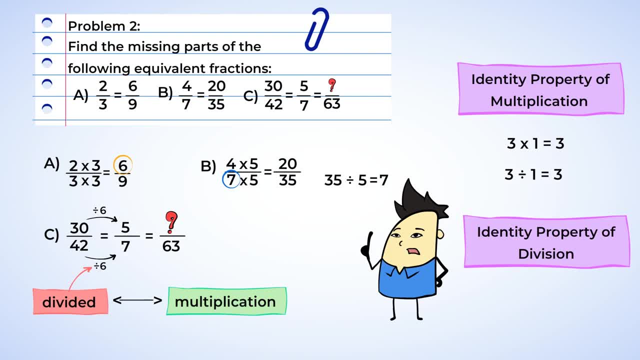 property of division. Any number divided by one is that same number. Okay, back to our problem. Now that we have five-sevenths, we can use that to find our other missing number. Okay, looking at the denominators, seven times what gives us sixty-three?